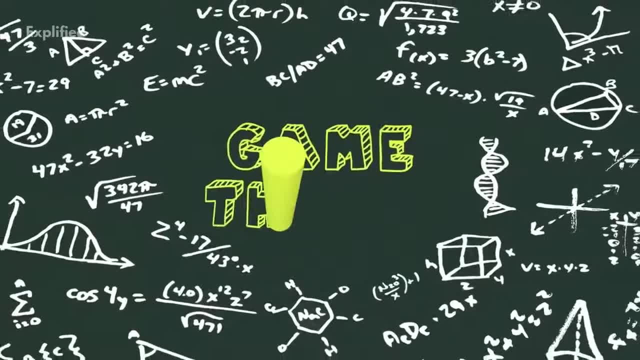 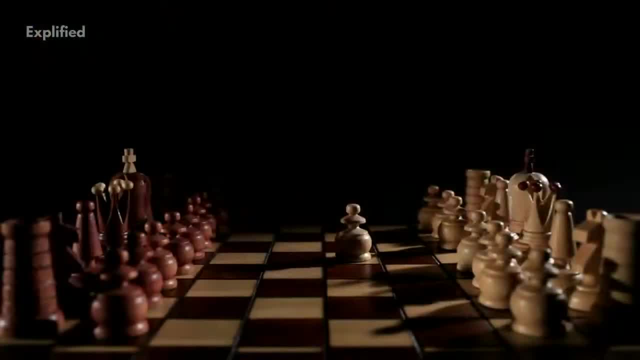 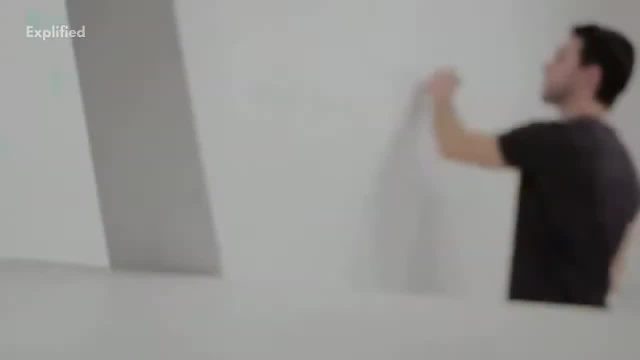 among rational players. The key to game theory is that one player's payoff is contingent on the strategy implemented by the other player. The game identifies the player's identities, preferences and available strategies, and how these strategies affect the outcome. The theory offers a wide number of applications in different fields, including economics. 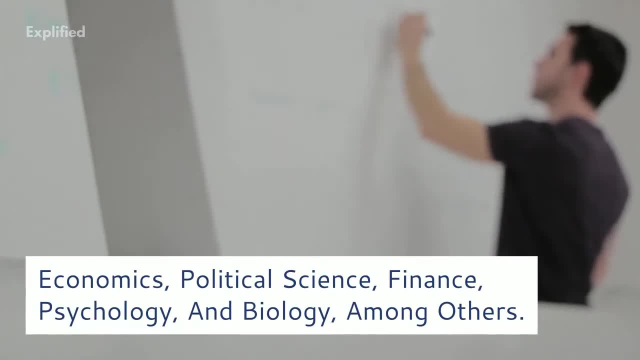 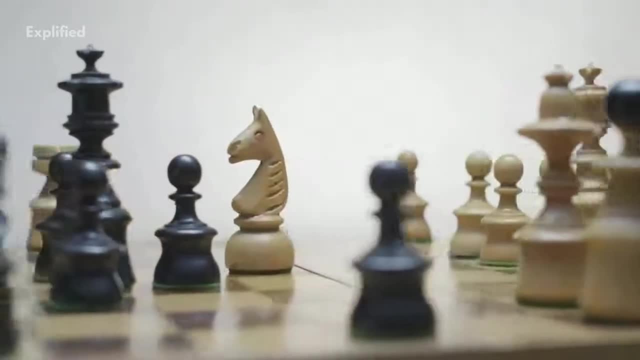 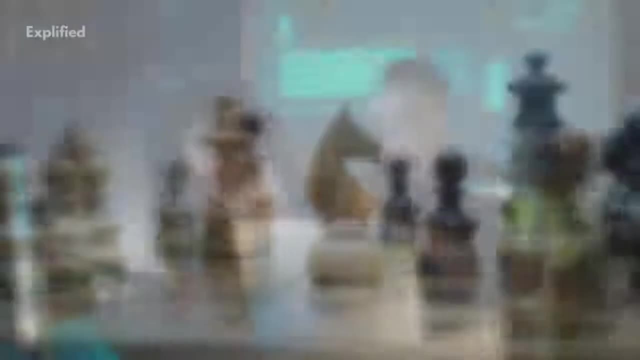 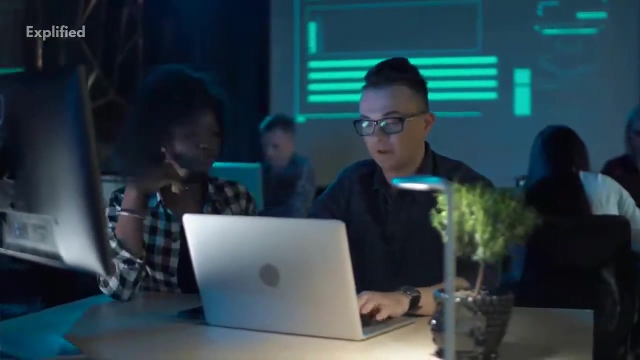 political science, finance, psychology and biology, among others. Any time we have a situation with two or more players that involve known payouts or quantifiable consequences, we can use game theory to help determine the most likely outcomes. Nash equilibrium is a concept in game theory that determines the optimal solution in a 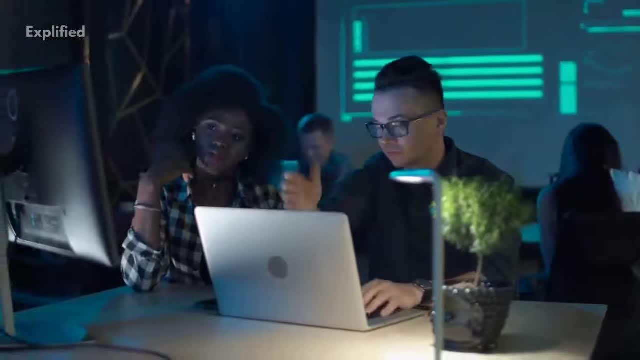 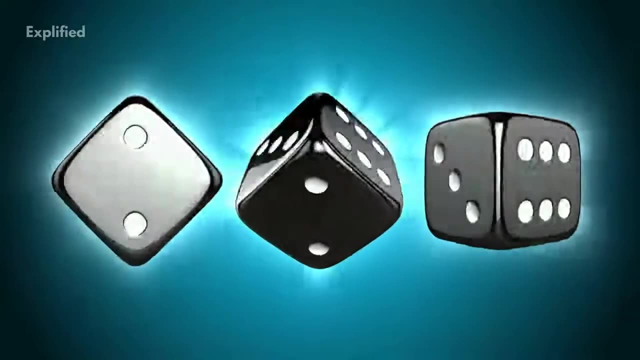 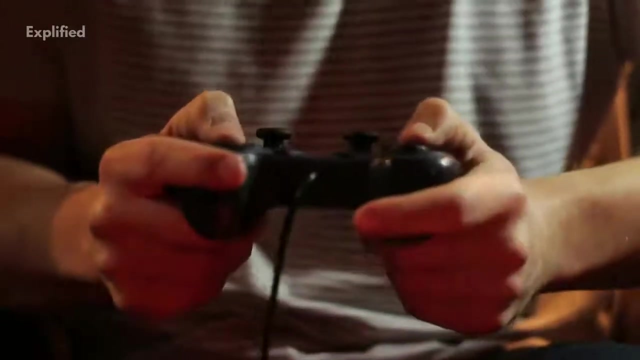 non-cooperative game in which each player lacks any incentive to deviate from his or her initial strategy. In game theory, a non-cooperative game is a game with competition between individual players. More specifically, Nash equilibrium is an outcome where the optimal outcome of 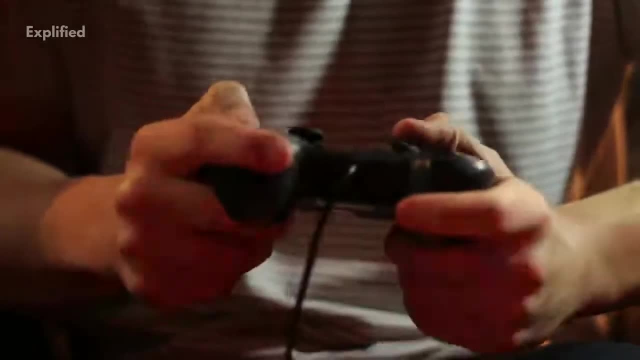 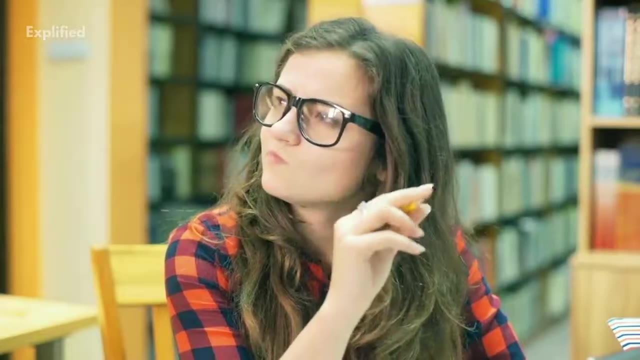 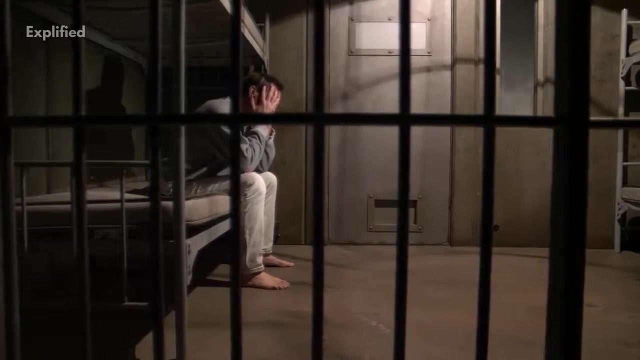 a game is one where no player has an incentive to deviate from his chosen strategy after considering an opponent's choice. Let us take an example to understand this. This example is popularly known as the prisoner's dilemma. Two criminals are arrested and each is held in solitary confinement with no means. 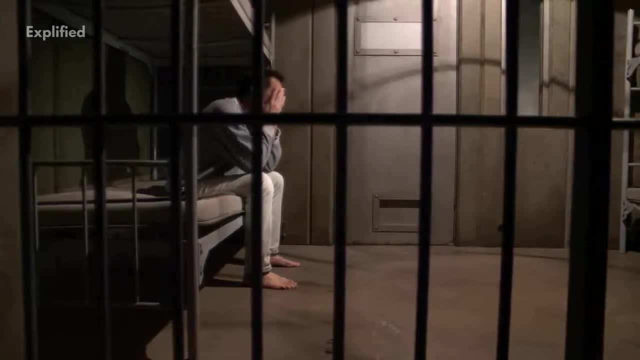 of communicating with each other. The prosecutors do not have the evidence to convict the pair, so they offer each prisoner the opportunity to either betray the opponent or take revenge on the other. The prisoners' dilemma is one where no player has an incentive to deviate from his chosen strategy after considering. 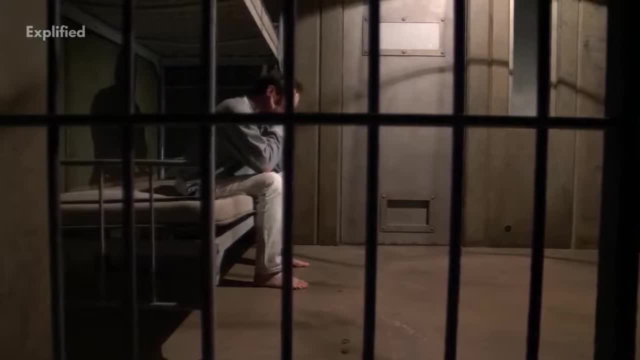 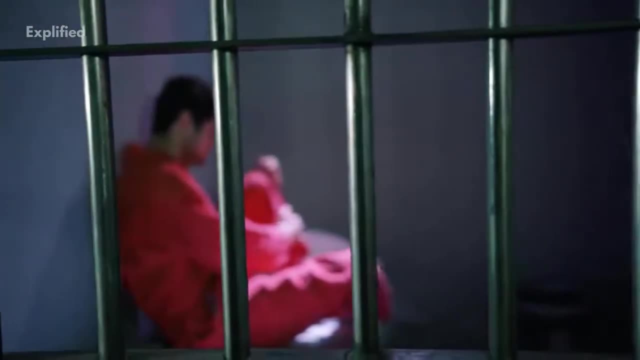 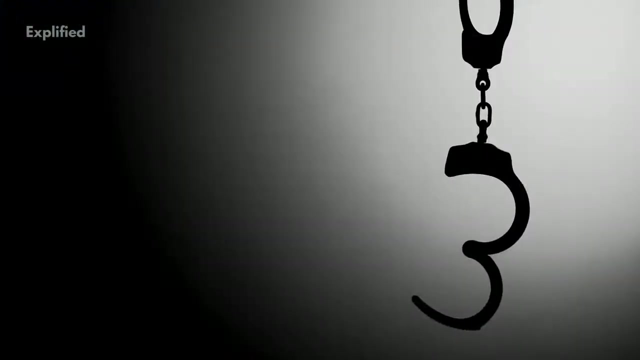 any other by testifying that the other committed the crime or cooperate by remaining silent. If both prisoners betray each other, each serves five years in prison. If A betrays B but B remains silent, prisoner A is set free and prisoner B serves ten years in prison. 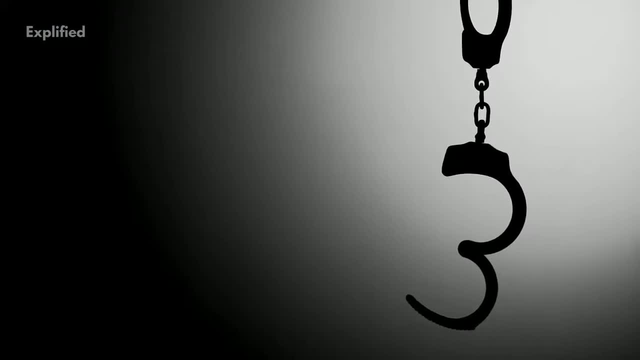 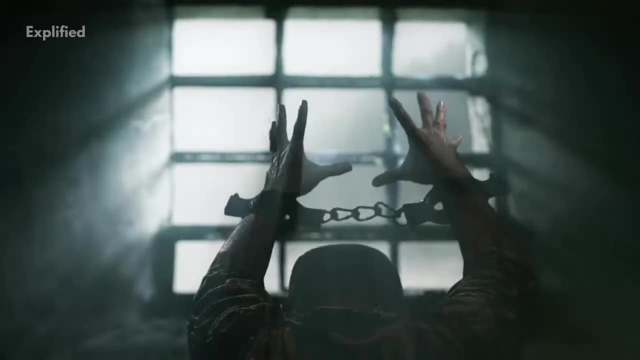 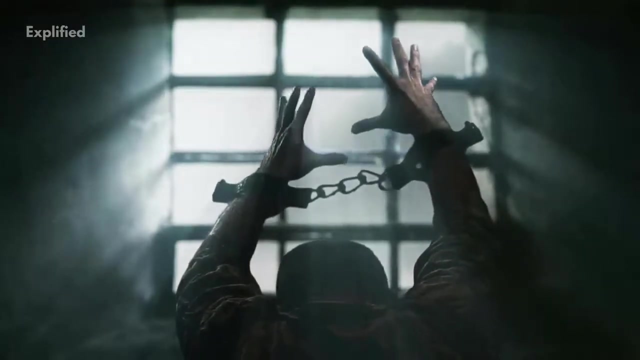 or vice versa. If each remains silent, then each serves just one year in prison. The Nash equilibrium in this example is for both players to betray each other, Even though mutual cooperation leads to a better outcome. if one prisoner chooses mutual cooperation and the other does not, one prisoner's outcome is worse. The concept is that in a closed